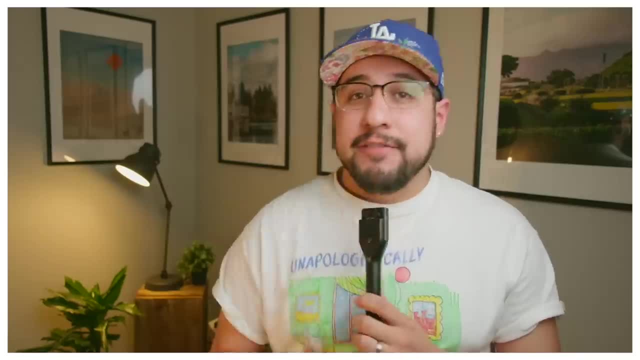 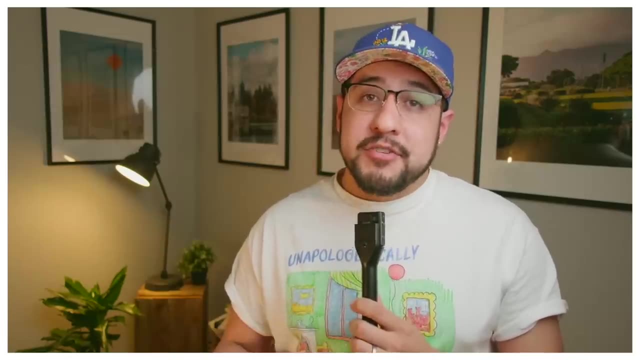 time I had one of these small cameras and say, hey, can you take a photo? I wanted something simple, wanted something easy, and I wanted something that I was hoping for would take great images, that I could do cool things with straight out of camera, And that led me to somehow finding 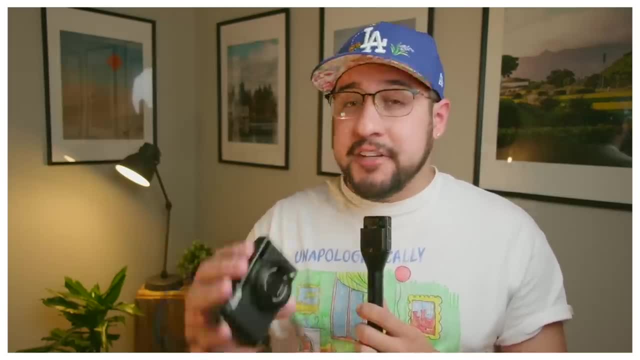 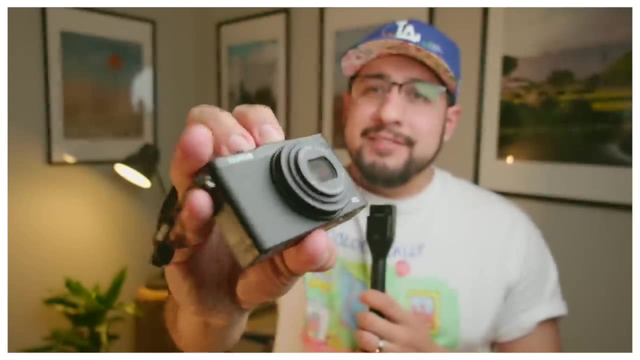 a camera I didn't even know existed, And it's Fujifilm's XQ2.. Now, this little camera right here, crate, crazy, great. I don't know what to say, for a couple reasons. Number one: this is an X-Trans sensor. 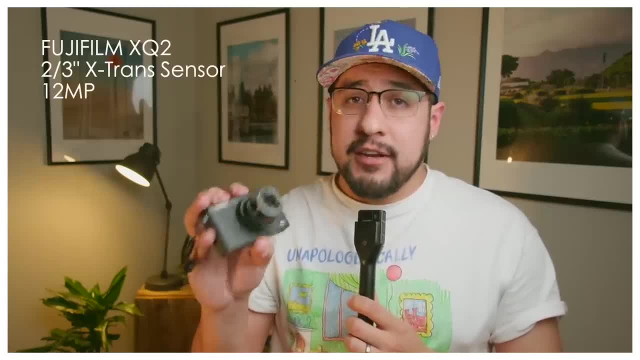 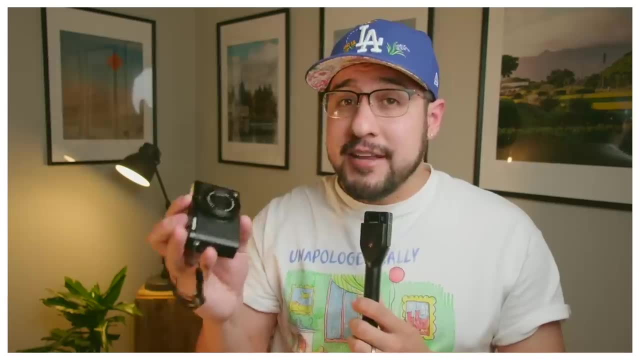 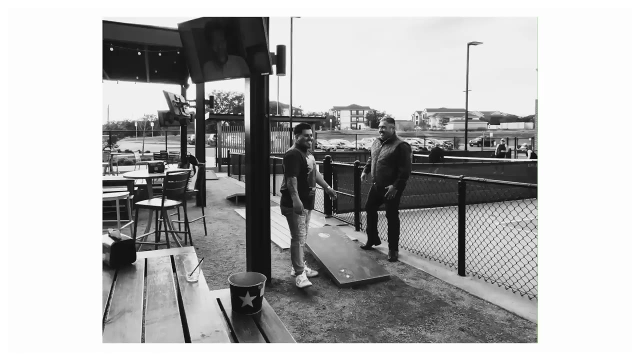 a two-third X-Trans sensor And for it being over a decade old, I got to be honest. the autofocus is really damn good and really damn snappy, Even in some low light situations. this thing is going to hit a lot. Number two: the lens is pretty great for the size of the camera. Couple that with the. 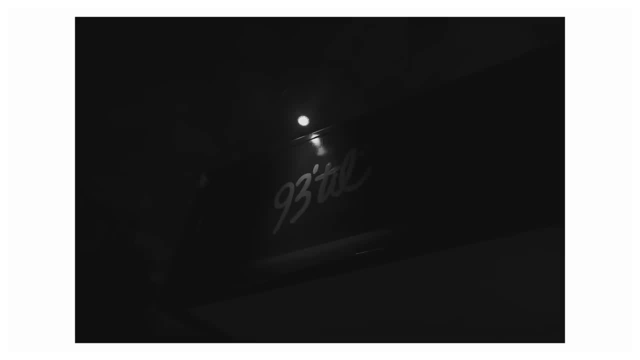 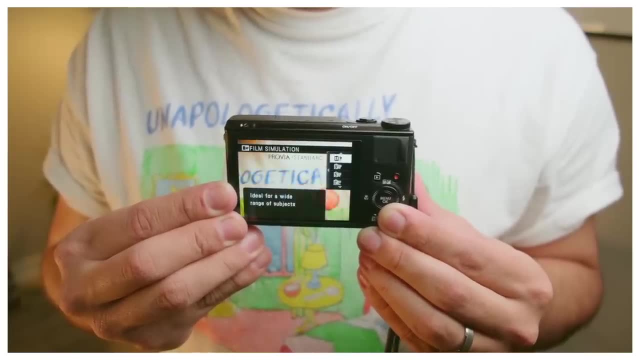 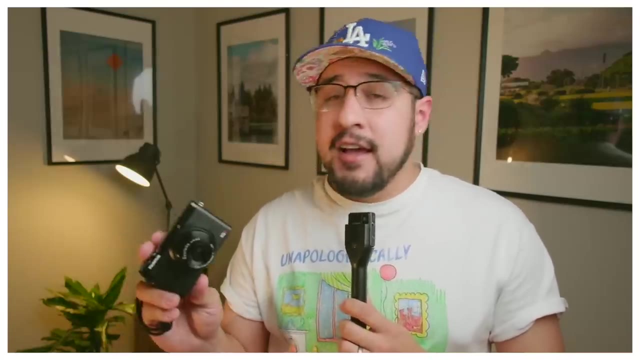 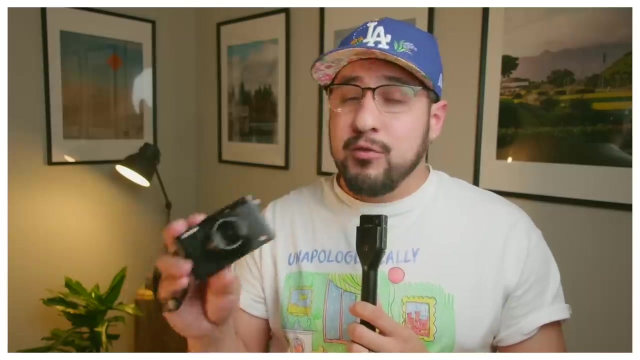 fact that it's got a lot of built-in cameras. Number three: it has a huge film simulation that you can put in. for this one You can put in a Portra 160, or a Kodachrome, or a classic film or film positive, whatever in the world. There are so many of them that are named For me personally, I like to use this for a T-Max film simulation. 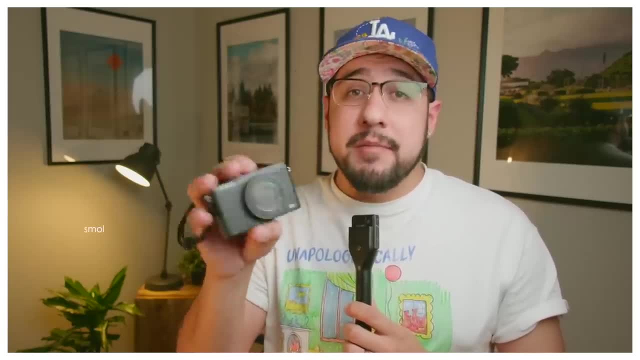 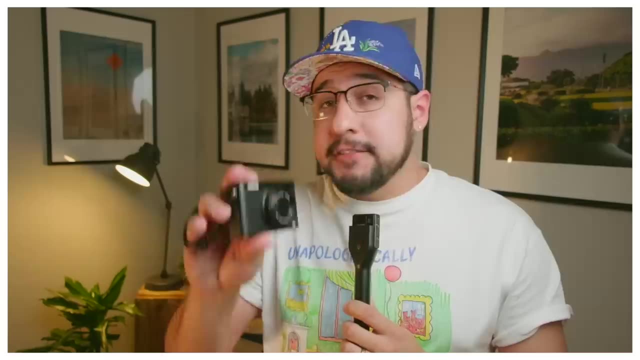 calculation. This camera right here is small- S-M-O-L small- and I absolutely adore it. I got it in really good condition And, let me be honest, I started searching for this camera and started looking online and people are selling this for $300 or $400.. If you see this camera after a day. 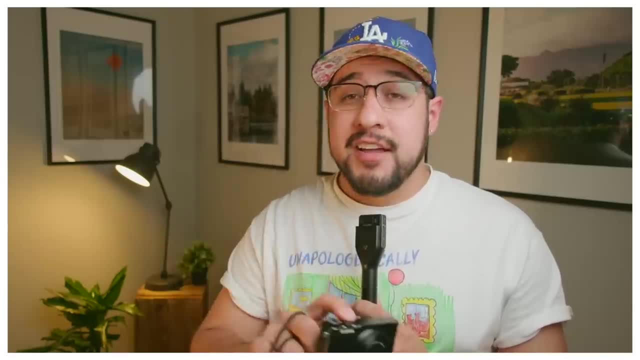 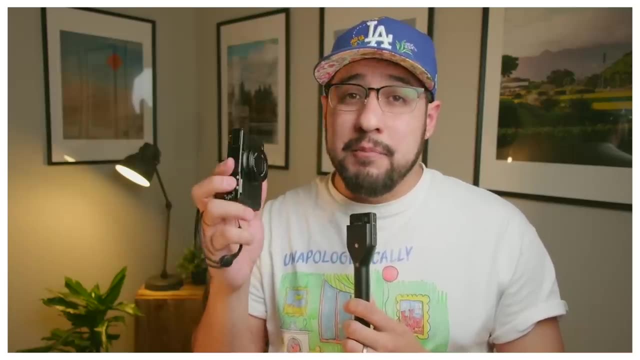 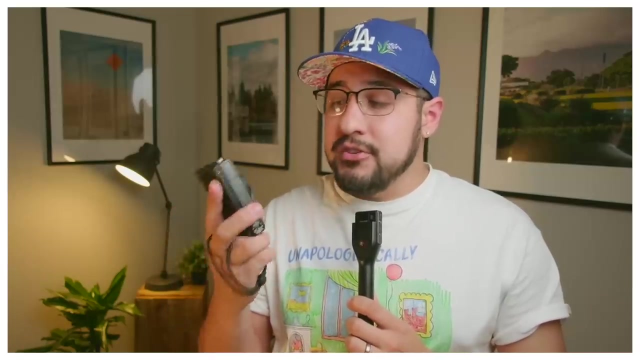 and you say I really want it and someone is offering it for $300 or $400, don't buy it. $200 for mint condition like this at the max, but most likely you're looking at a camera that is no better for the price of $150 and whatnot. But it's great. I really am enjoying this camera. so 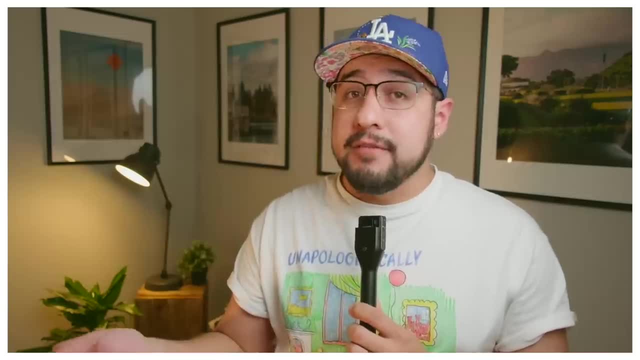 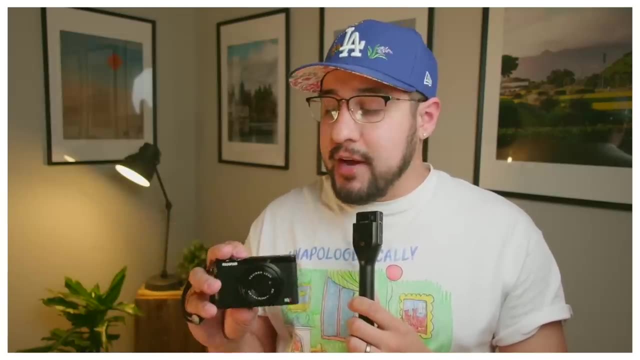 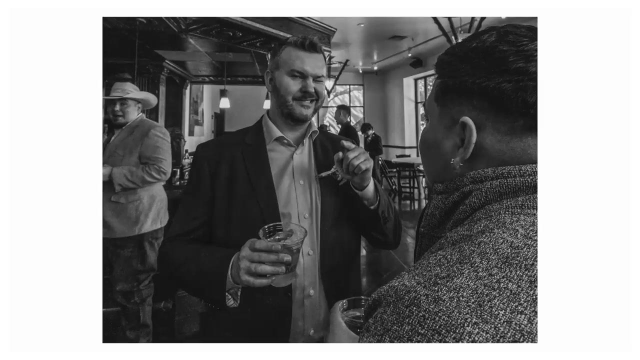 much so that there were so many situations where a Leica would have been more beneficial. With my 35mm f1.4 Voigtlander lens on there, it would have been a lot better for low light situations. But during my wedding, which I was taking photos during and before my wedding- funny enough. 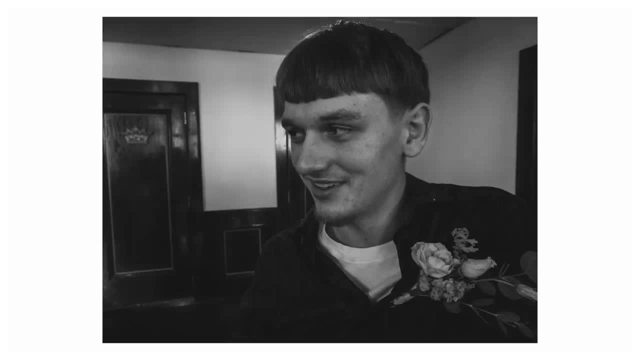 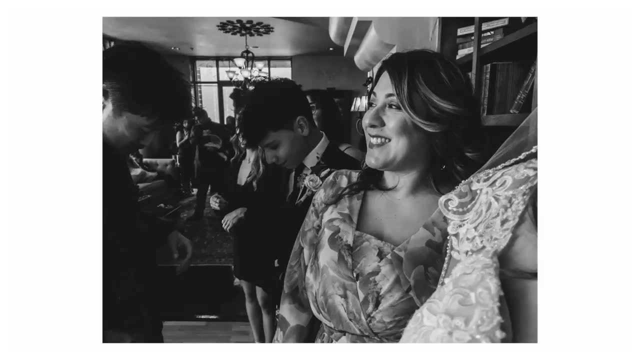 I had this in my hands and I'll show you some of the photos that I took while I was doing that Or just during my honeymoon, even some time before and in between with friends over here at Bright Coffee in San Antonio. I just really enjoy this camera. I enjoy the images that come out of. 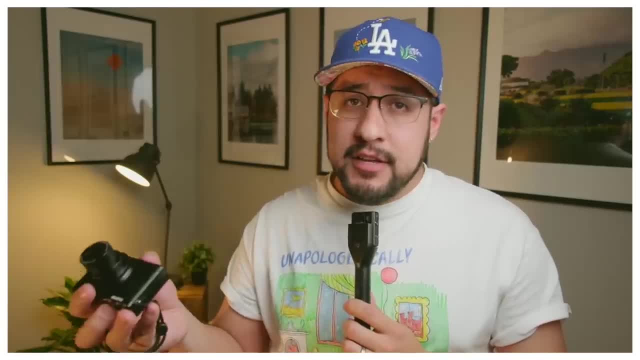 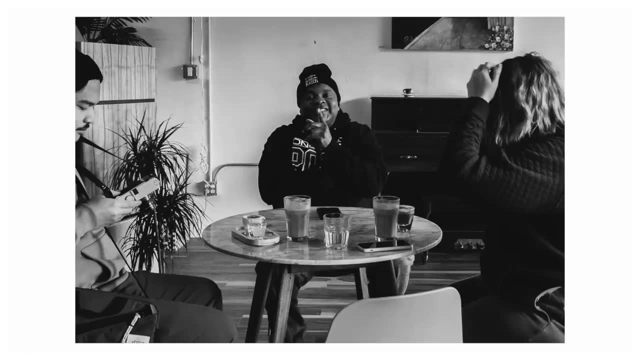 it More than anything. I just liked carrying it around, And that's a big deal. See a lot of us. we get a camera, sometimes for the features, for the sex appeal, for the look, for the notoriety. 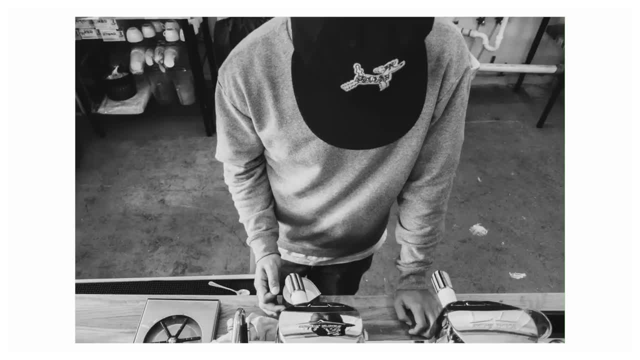 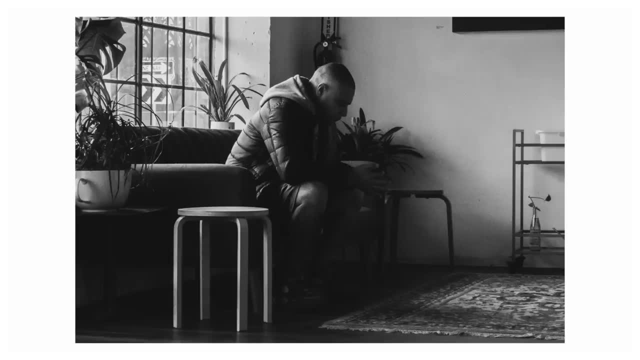 You see, the good thing about this little camera was number one: it was cheap as hell- I mean, honestly, a steal for the price that I got this at. And number two: it's good enough, And a lot of times we're so just stuck on the idea of 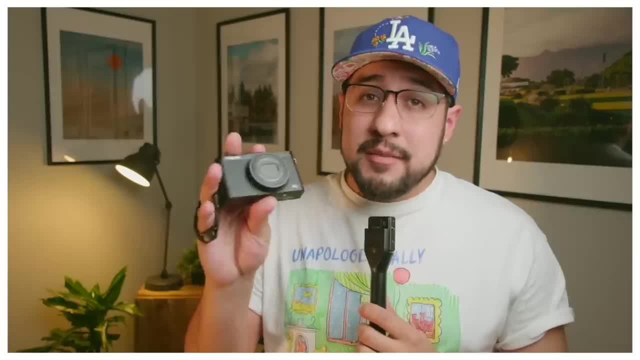 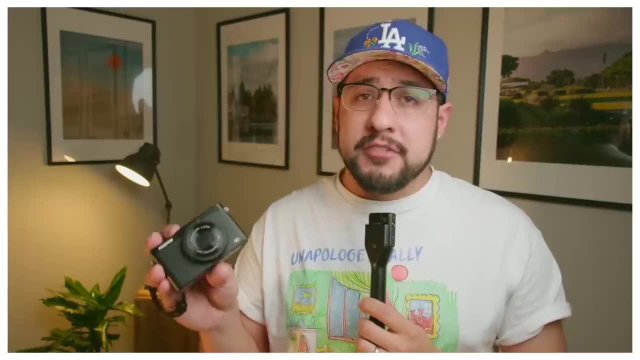 perfection, perfection, perfection whenever it comes to cameras, when sometimes good enough is always going to be good enough. This camera does not do fantastic in low light, It's not going to take the sharpest images ever, And this is not a replacement for a Ricoh GR3, an a7 III. 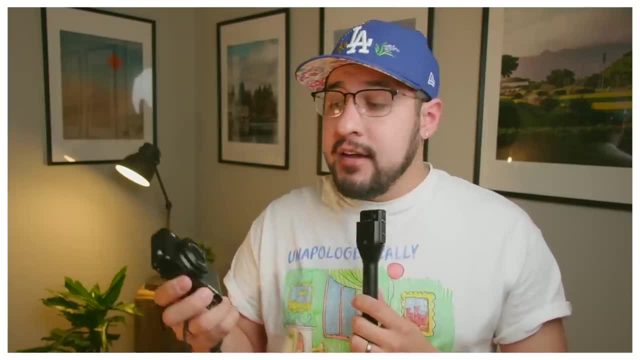 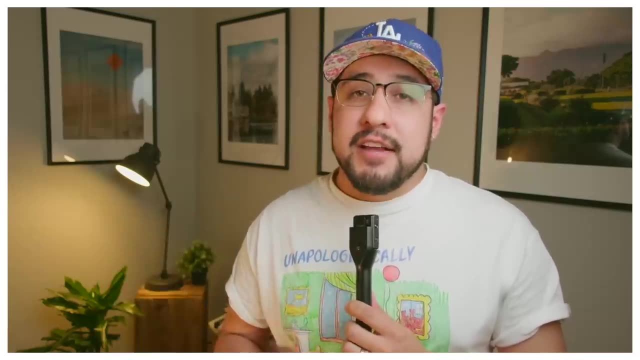 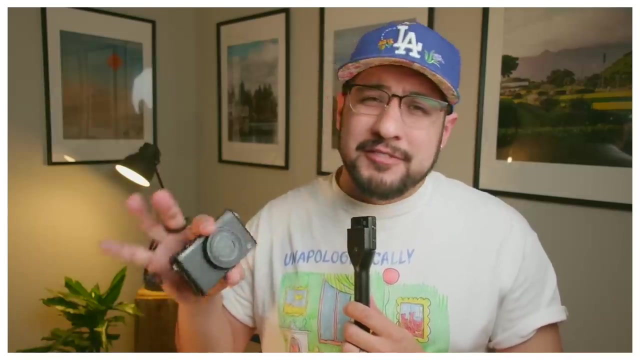 anything you're using right now for professional work, And I think that's where the beauty of not meant to be replacements And right now we're so fixated on things- when the Ricoh GR3 came out and GR3X, when the X100V came out and we have the Leica Q series, in a sense it's still big. 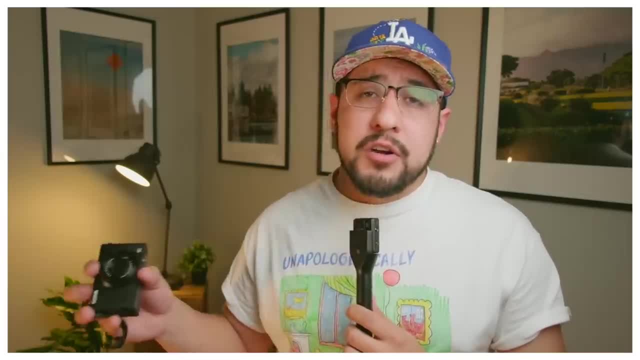 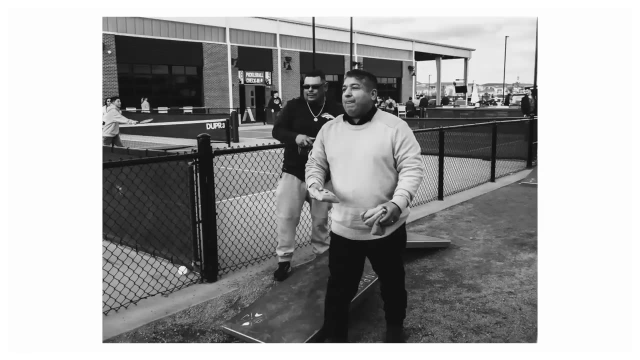 The Sony RX1R or whatever in the world, RX1R Mark II. those cameras are small but they're still kind of big. but they're built and have the sensor and technology for a lot of people to replace a flagship camera for them, for their needs. 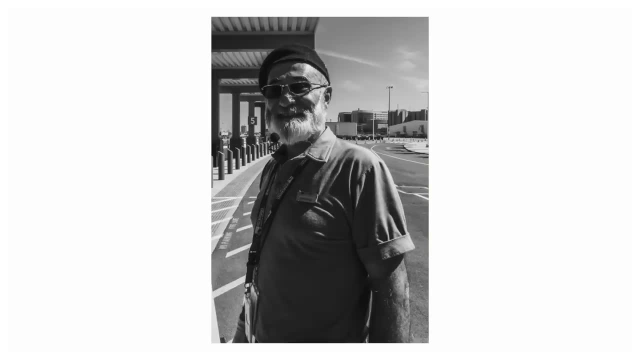 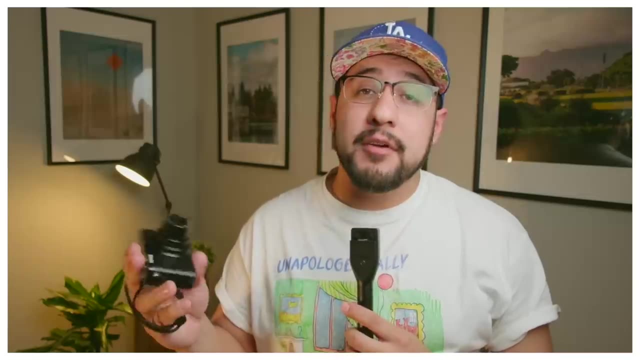 This camera's not that, and it was never trying to be. This camera's about being fun. This camera's about being in the moment, And this camera's about being able to get the hell out of the way the moment you want it to. Now this camera is packed with quite a few features, Most notably 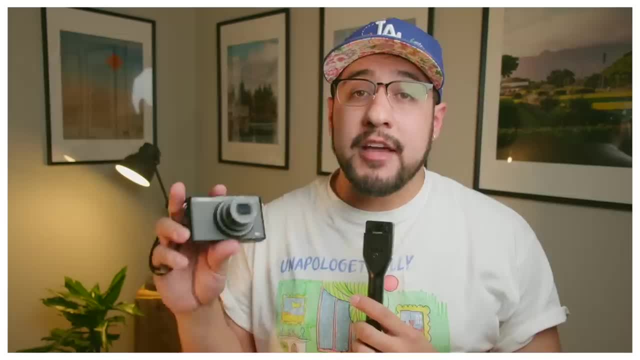 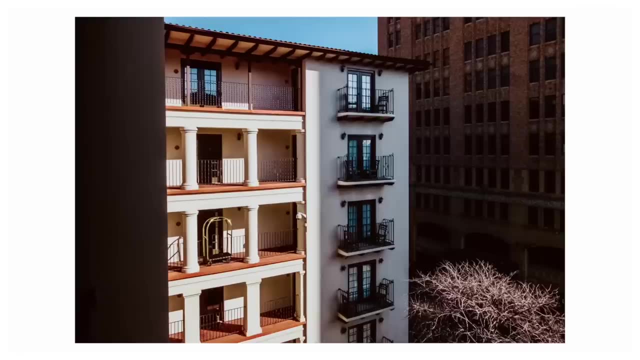 it's those film simulations that I mentioned before that are in here that allow you to have amazing straight out of camera JPEGs. Again, I shoot this primarily, though, as a monochrome camera, but the colors coming out of here are really great. The grain, because it has an X-Trans sensor. 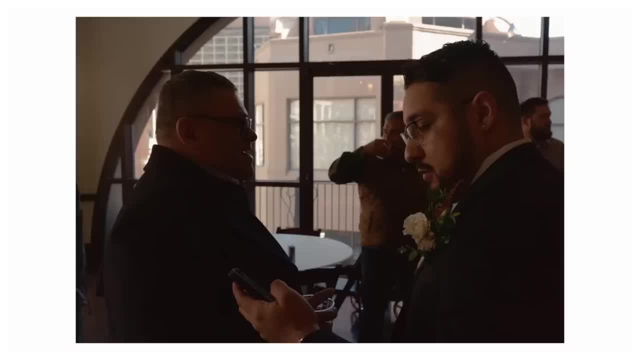 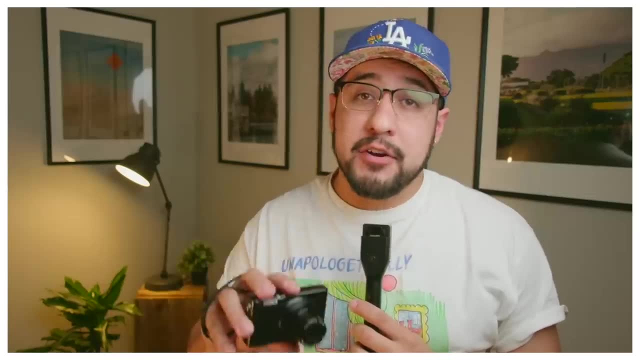 is nice and random, so it actually does feel like film, Even though if you go above ISO 400, the image falls apart pretty quick. Nice black and white, a nice cinema curve will fix every single thing. The detail is still there in the highlights and 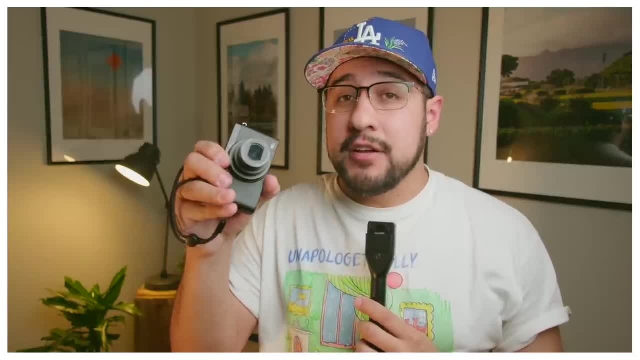 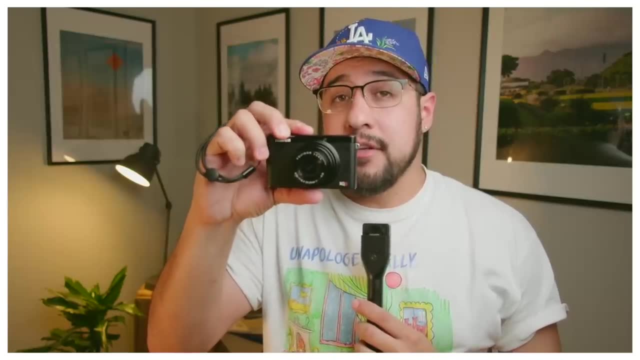 the shadows, and I really, really like it. It comes with a nice little ring on here that can do a couple things. You can assign it, like I do, to zooming in and out, as well as this toggle rocker on top to be able to zoom the camera in and out. It has a nice little area right here Boom. 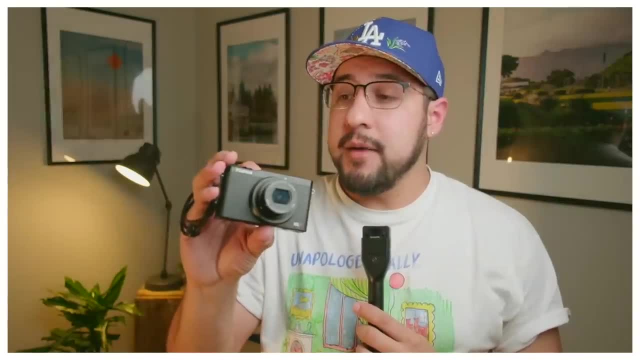 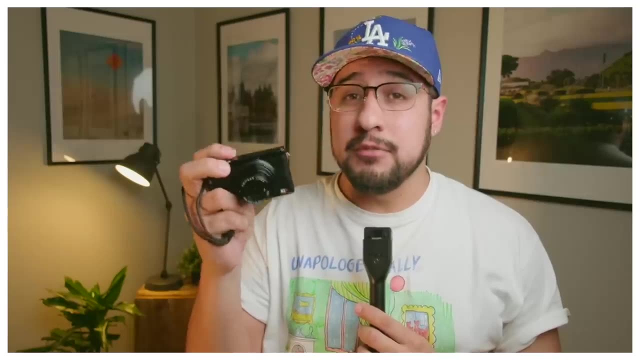 you got a flash in this camera. That's pretty sweet. It also comes with a few things: a PSAM dial on top- Very nice for those of you- A macro mode that is an actual macro mode. I really like that. It gets hella close whenever you have it on macro. 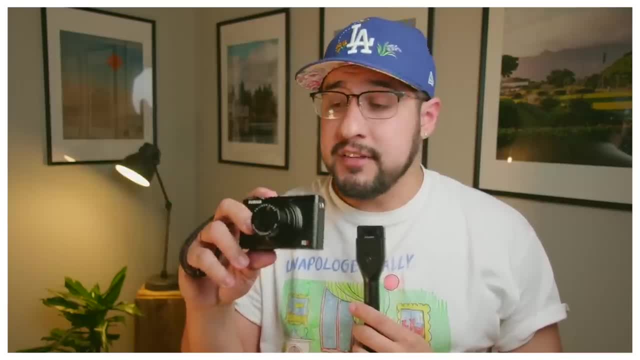 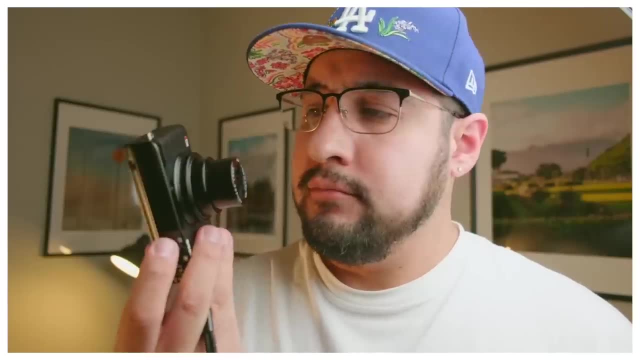 mode. It has the ability to record, which is nice, but the image quality sucks. But, more than anything, it just gets out of the way. Whenever I'm shooting this, I shoot this on manual and I adjust all the settings. I make sure things are right. I adjust my depth of field to what I want. 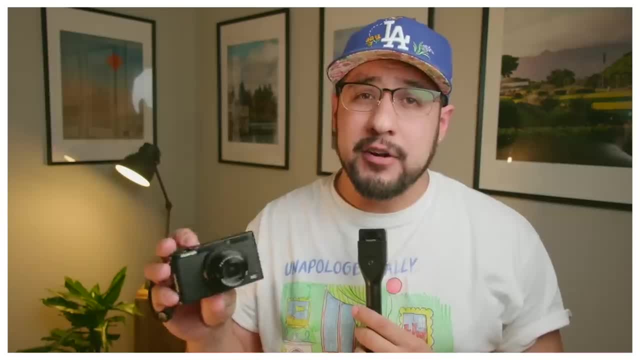 it to be F8,, F11,, F8.. You can adjust the depth of field to what you want it to be. You can adjust the depth of field to what you want it to be. You can start to fall apart in the image, But F5.6. 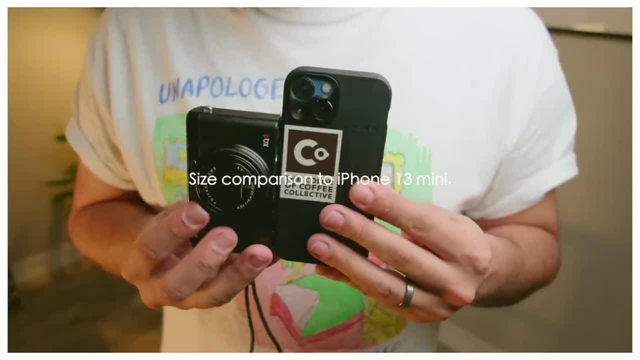 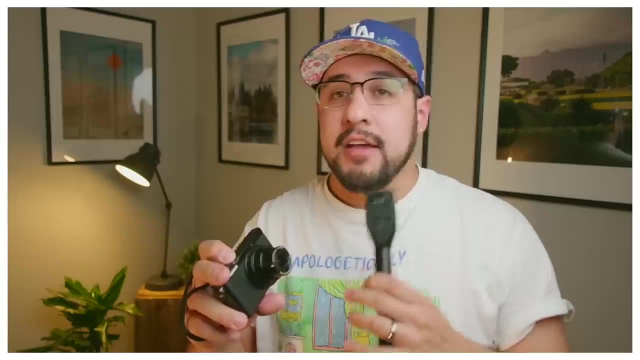 and below, the image is always going to be super sharp And I just start shooting. But if I want someone else to shoot this, if I want my fiance, my wife- so I just got married- If I want my wife to shoot this, if I want a friend to shoot this, a family member who doesn't know anything about, 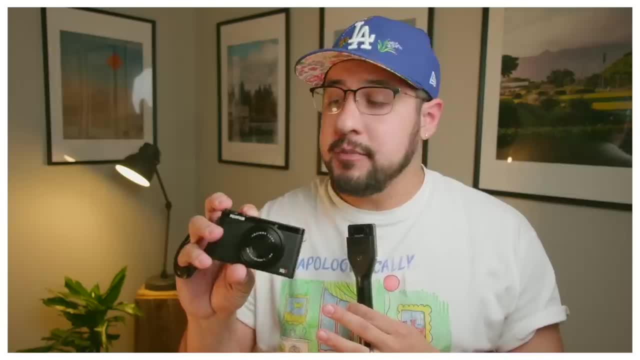 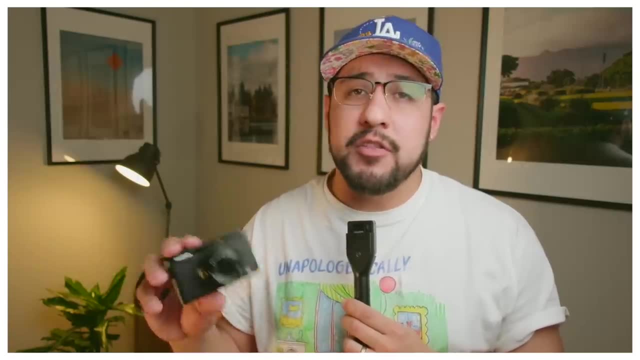 cameras. all I got to do is switch over to the SR plus mode, which is basically like an automatic on steroids, And they're able to take a photo. the exact same settings I had, but the camera does all the work. It balances for highlights. 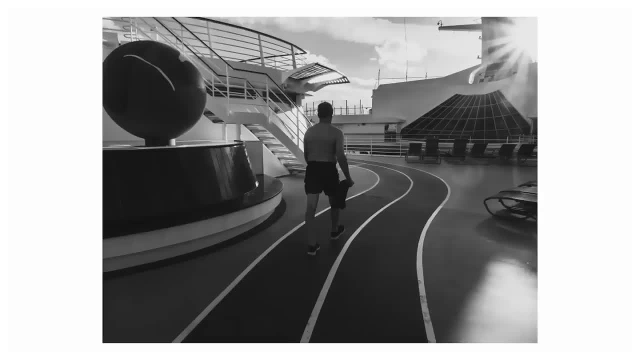 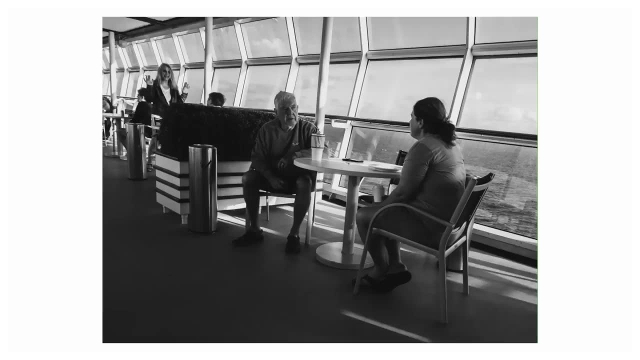 Takes a good photo. IBIS is built in. You're not going to be able to miss having the moments you want captured with this camera, And I think that's what I love the most about. it Has continuous shooting, I believe up to three frames per second, but didn't need that. This is a fantastic camera. 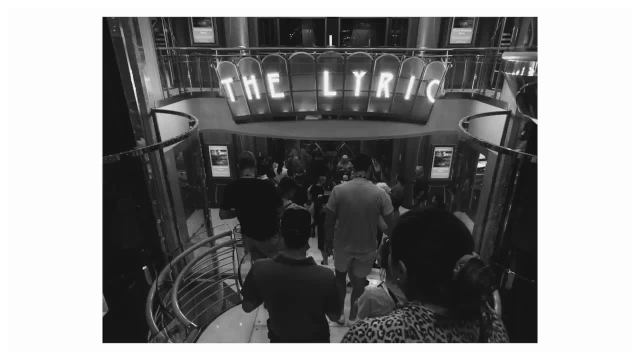 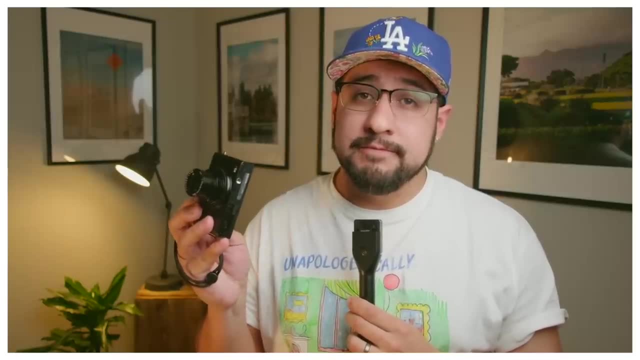 Just pop up out of your shirt pocket, take a photo, just like I did there, and close it. That's it. That is literally the response time Here. it is open And I just took a photo. It's very, very quick Again if you turn off pre-focus on. 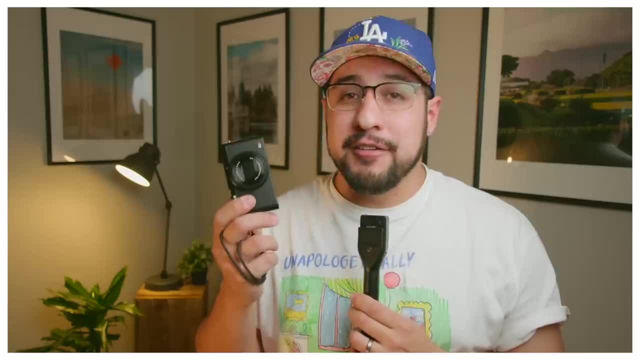 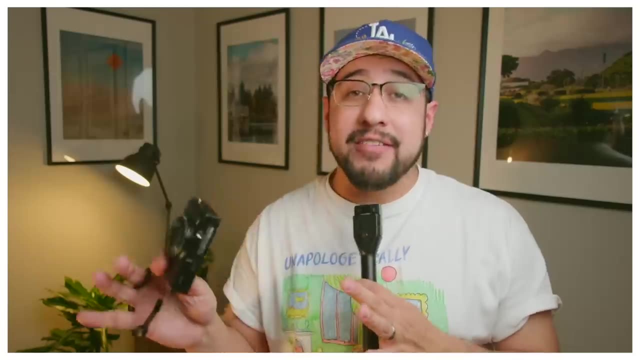 this. it gets even quicker. A fast camera for the size and for the technology at the time- Amazing. I've not even done an update on this camera, Not even sure if they have an update for this camera. and it's just that damn good. And little cameras like this, I think, are very, very necessary, Even. 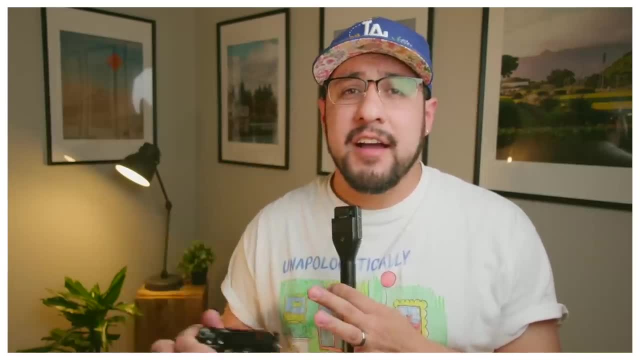 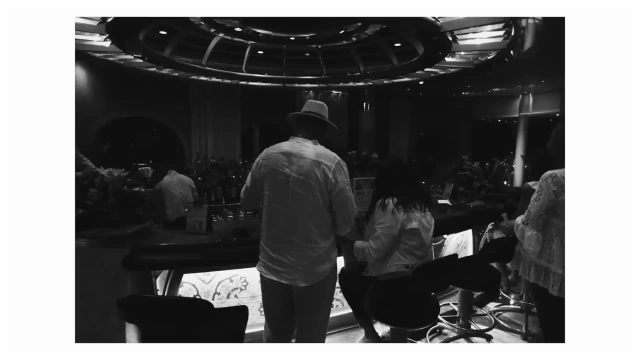 if it's not this one. you see, for the longest time in my photography journey, cameras were tools, tools, tools, tools, tools, And I have to create a great image, a great image, a great image, The older I get. 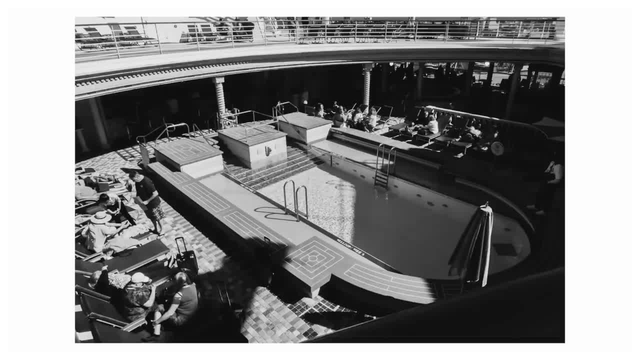 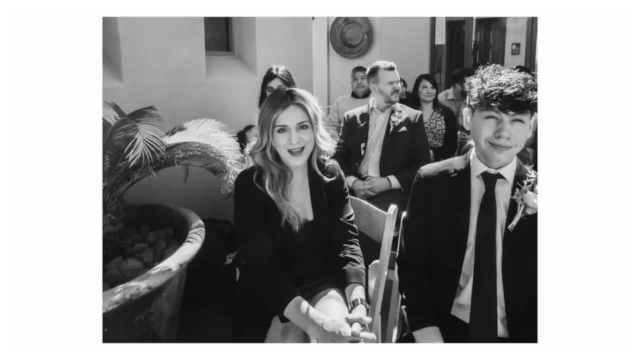 the more people that come and go out of my life And the more moments happen where I really want to capture these memories, the more I start having times where I don't care. if I capture the memory because I want to be in it, I don't want to change anything. I don't want people to look at me. 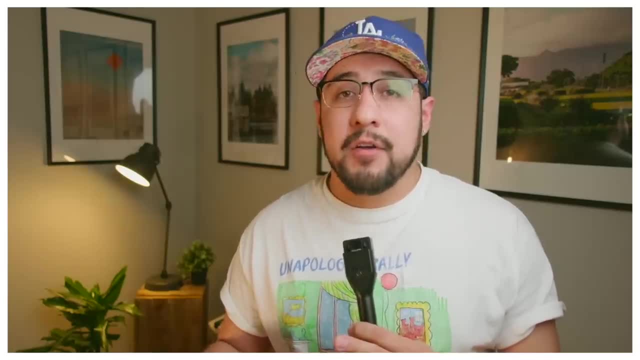 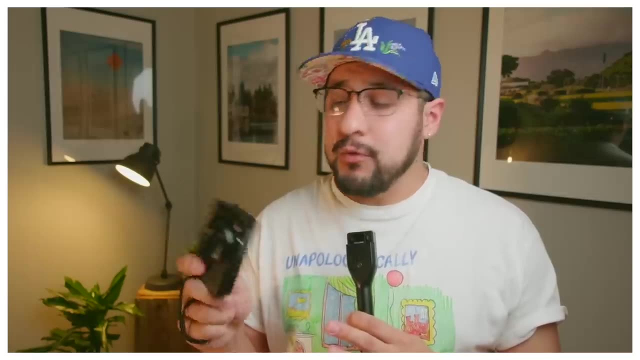 I just want to be here, And even more than that. I don't want to have a big camera on my neck, I don't want to be just the camera guy, I want to be participating. Little cameras like this, whether they're great or they're bad. a Ricoh GR3,. 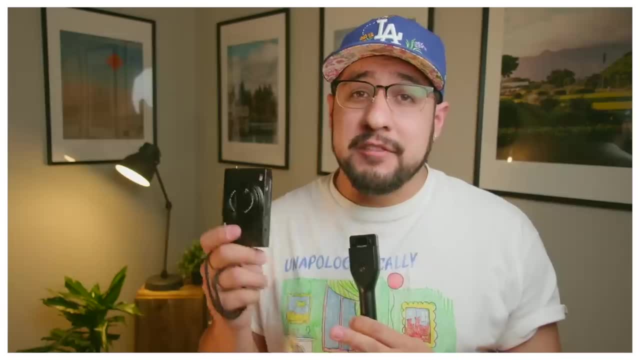 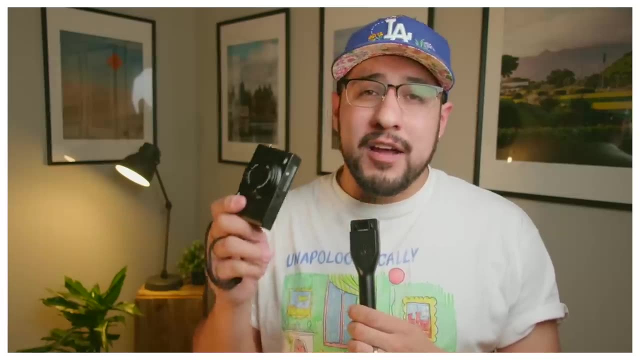 I don't want a bad camera to have, just because it's really good. That's a fantastic camera if they could fix that back, damn scroll wheel. But little cameras like this are so great because they give you this weird ability to be able to be a part of a moment even more intimate. 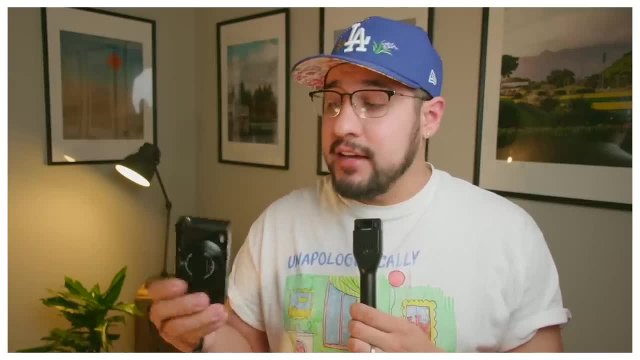 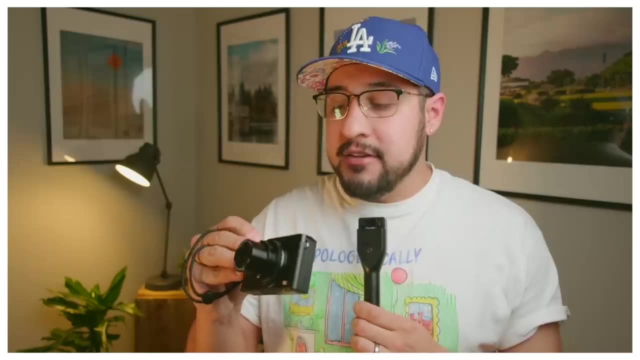 than any other camera, not disrupt anything and still being able to decide: do I want to capture or not? If the image is blurry out of this, I don't care. If the image isn't the sharpest out of this, I don't care If I blew some highlights. maybe was underexposed a bit. 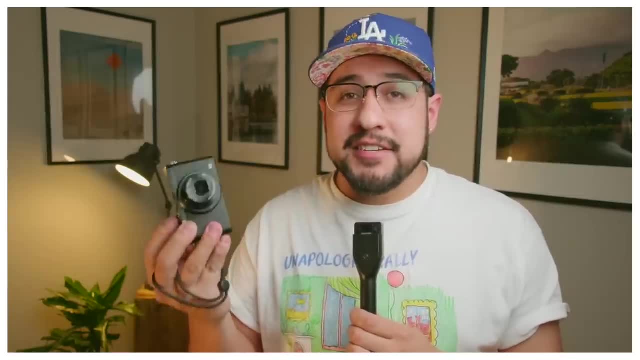 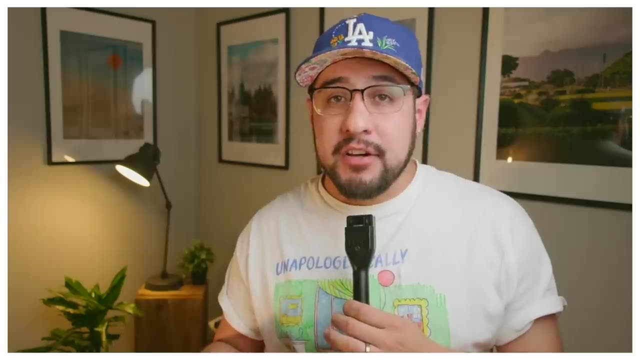 I don't care, Because, at the end of the day, this is designated for just capturing the moments that I'm hoping I don't lose. You see, in between all of our spec talk, in between all of our gear talk, in between all of our lust and what's going to come up next and what's going to be the next. 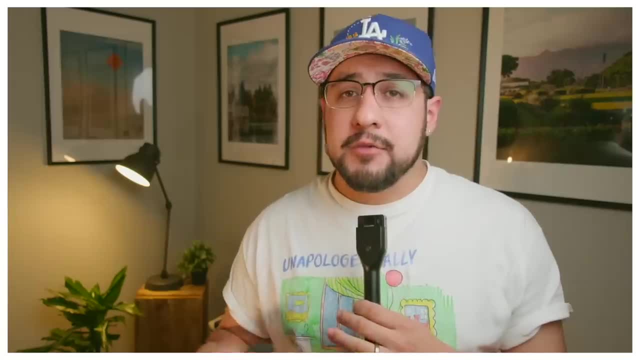 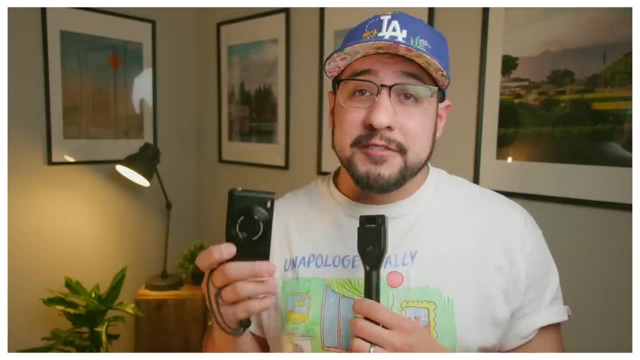 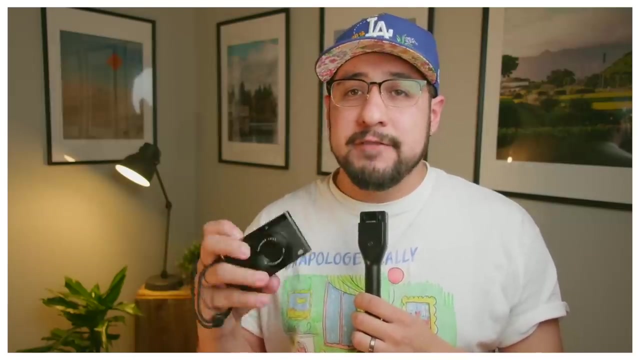 camera up. what's the new sensor? what matters at megapixels, what matters with this, that and the other? there are photos to be taken and there are moments to be shared, And that's where these cameras step in. XQ2 does a fantastic job of that And, honestly, it kind of upsets me that Fujifilm continues. 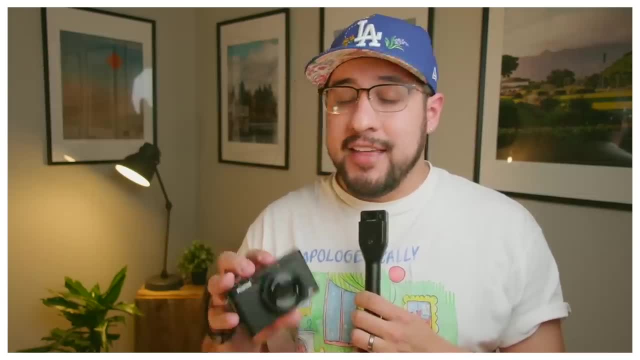 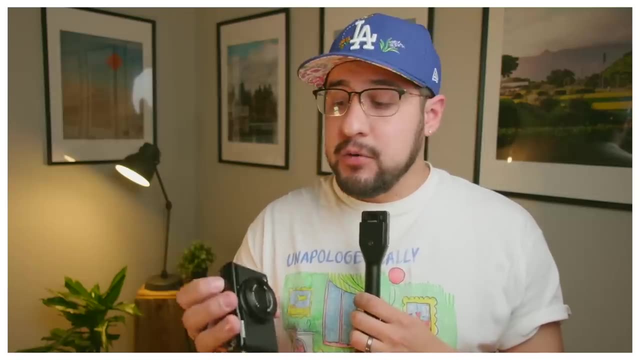 you know, as you look down the line with all the cameras they've made, they really don't like these small, pocketable point and shoot cameras, whether it's the XF10, the X70, 28 millimeter fixed focal lengths or this one right here with the four time optical zoom that gives you about an effective 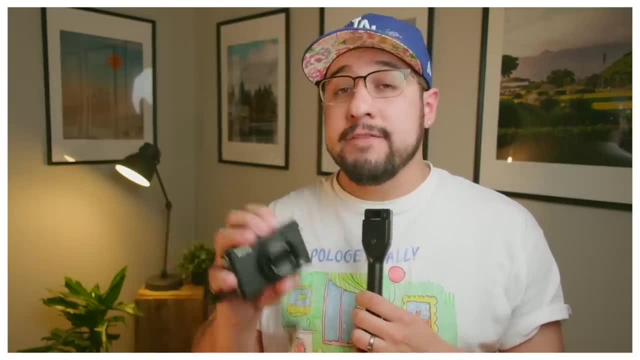 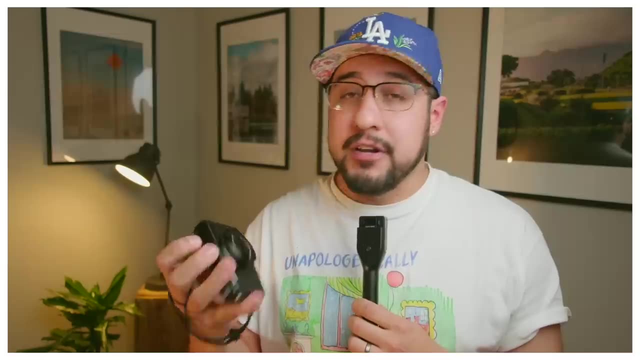 cropped focal length or field of view of 25 millimeter to 100 millimeter. You know they can get f1.8 to f4.9.. At 25 millimeter you can get f1.8 and the bokeh is pretty good, but I don't. 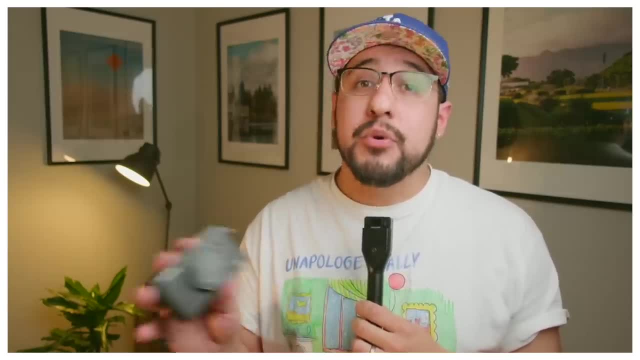 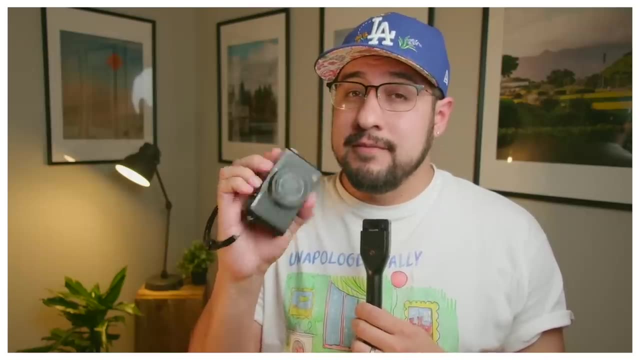 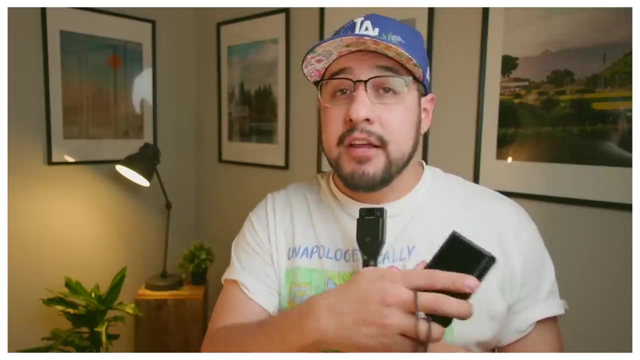 think I've ever shot this thing below f5.6, unless I'm in supreme, supreme dark conditions. But even then this flash works pretty well. It's also pretty fun to knock up Nice. But it's lightweight, it's pocketable, It never got in the way. It's something that Shelly could carry and work with. 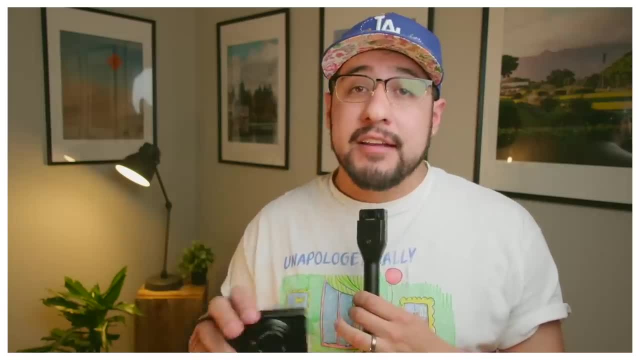 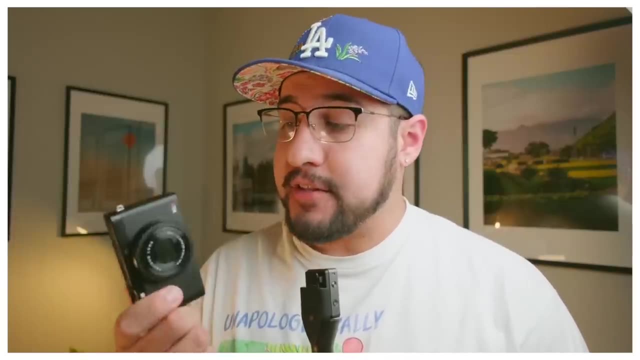 It's something that I could shoot and do all my street and candid and sneaky photography with. It's just a good damn camera. A couple of things I forgot to mention in the first part of this video about this camera is: this is an X-Trans sensor camera. It's a two third inch sensor camera. 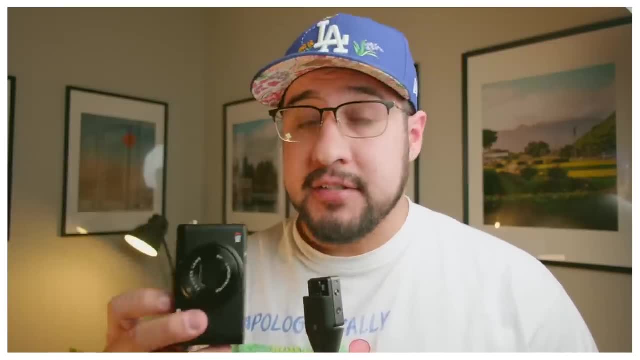 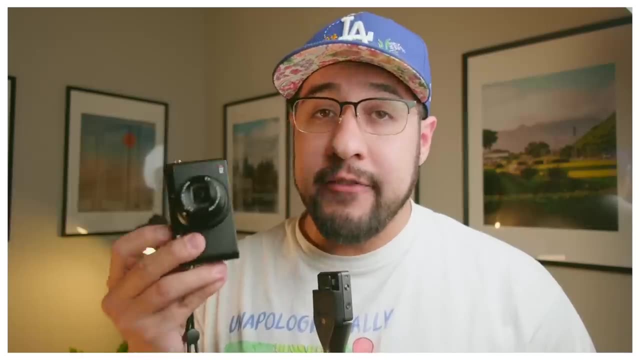 similar to what your smartphone has, but it's still X-Trans, And this means a couple of things. Yes, you're not going to get the best low light capability out of this, but because an X-Trans sensor, you're going to have a randomized grain pattern, which means the grain is going to look. 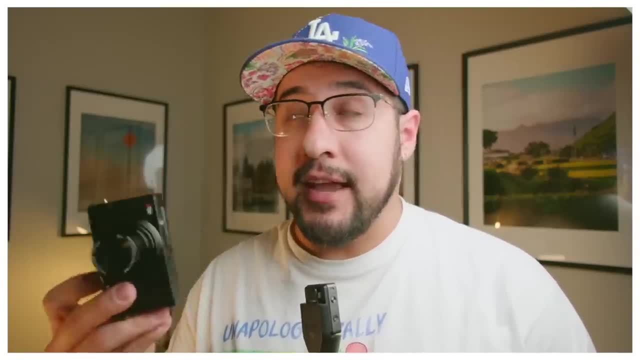 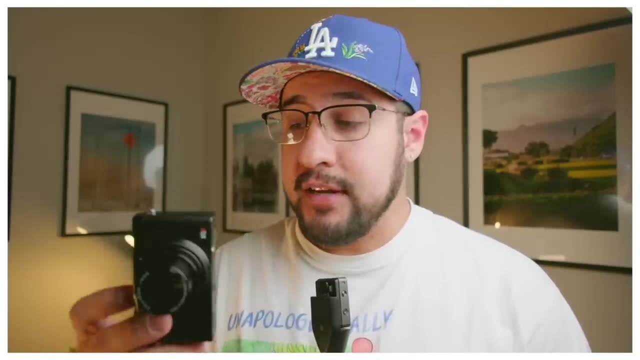 more akin to something you'd see out of a film camera, giving you a- I hate to say this- a more natural look, especially whenever you couple this with a black and white JPEG style shooting, It's going to be great. It's going to be fantastic And, again, that's one of the benefits of the X-Trans. 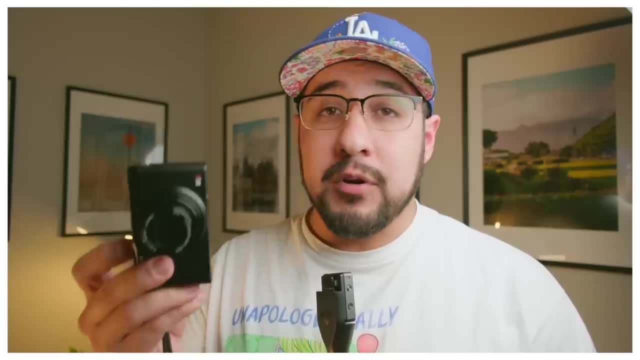 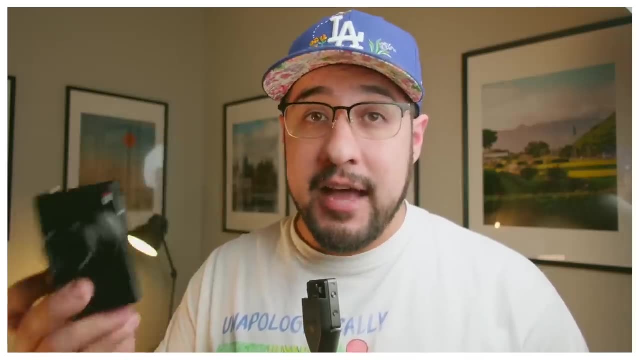 sensor. You get all these amazing colors that come out of it, but even more than that, you get kind of some makeup whenever it comes to lower light. You're still going to be able to keep the detail that you're missing out on because a smaller sensor and you're going to have a grain pattern. 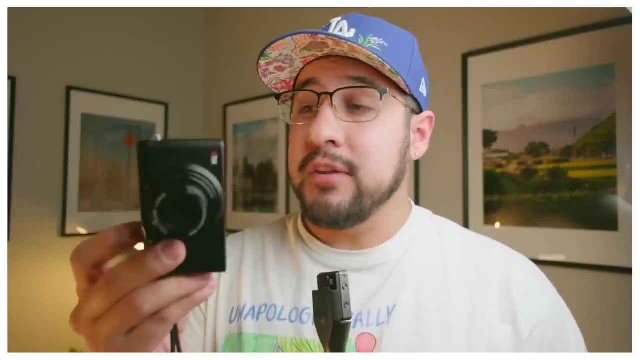 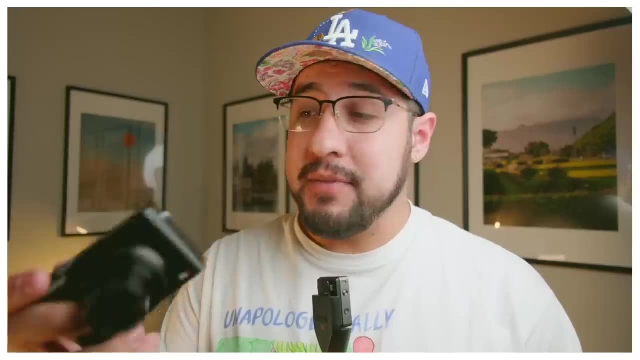 that is more pleasing and natural to the human eye, And even more than that. this camera is, just because of the size and just because I mean everything's intuitive. The buttons are where they need to be, And someone with a large hand like me shout out Lonnie George and the large 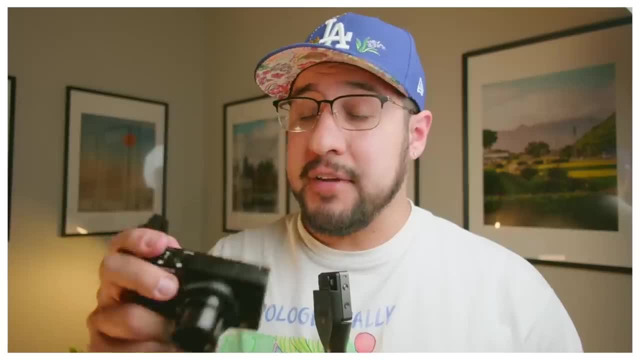 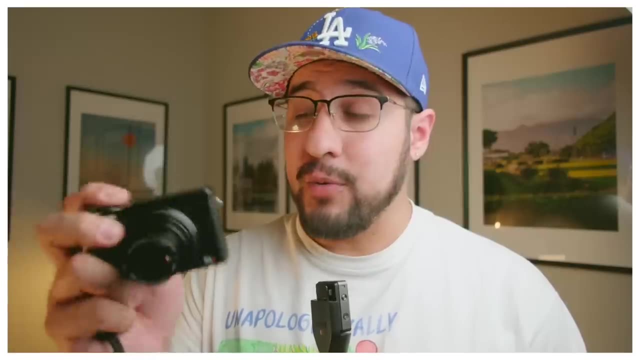 hand gang. Honestly, everything is where it needs to be. It's got a nice little grip on the back. The ergonomics are just fine. Again, with the IBIS coupled in it, it's a really good all around camera for just point and shoot usage. Low light, okay-ish light, really great light. 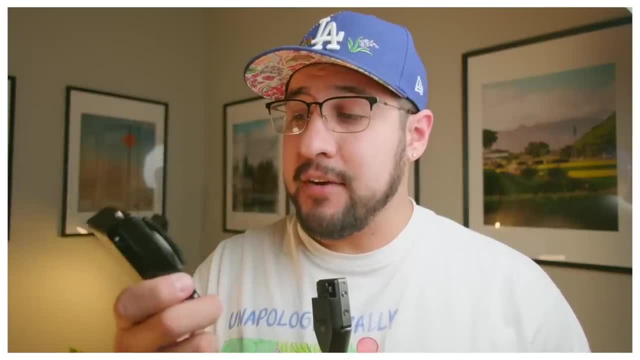 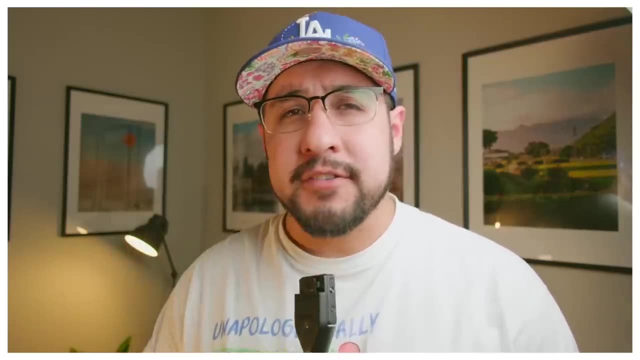 Now I will have to say this: even though this camera is as fantastic as it is, I don't think it's for everybody. but speaking of something for everybody, let's hear a word from our sponsor. Oh, hi, there, Didn't see you. My name's D. 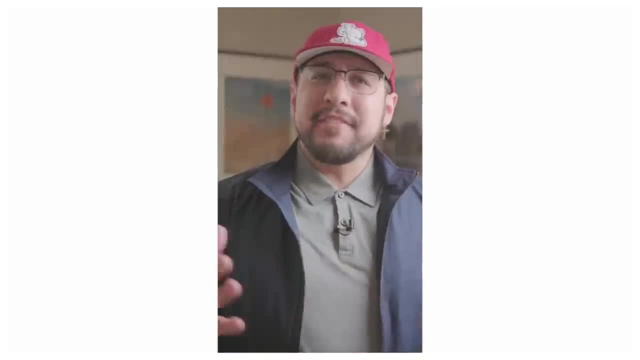 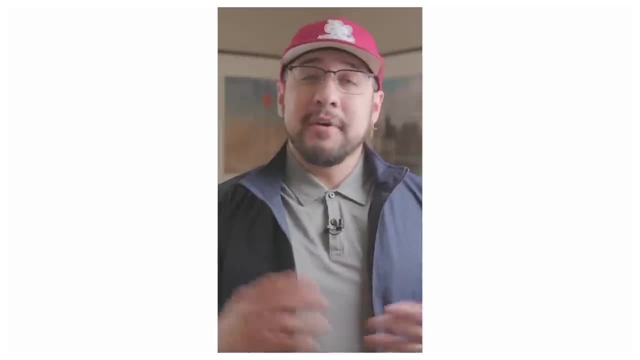 and, aside from being an avid reader, I'm also a Cuts ambassador. You may be thinking to yourself: you, you're a Cuts ambassador. I thought Cuts was for the handsome, beautiful people of the internet, and you're darn tootin' it is, But now, thanks to a new initiative, Cuts is allowing. 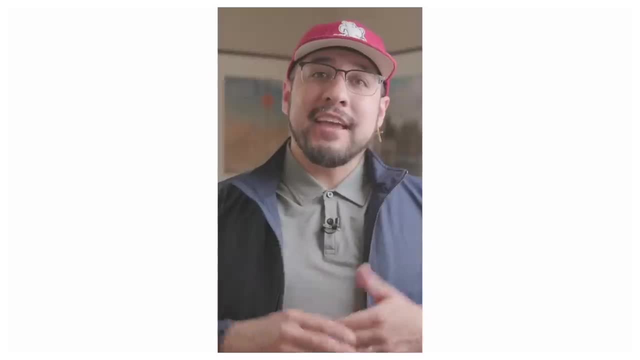 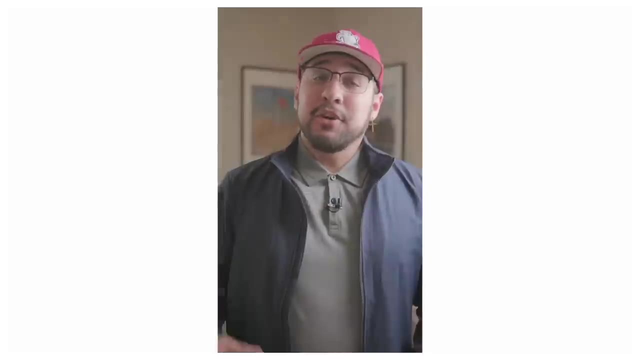 average everyday regular people like me. to partake in their amazing, well-engineered clothing feels good on your body but makes you look damn good in the process, So it doesn't matter if you're me or if you're one of my fellow Cuts ambassadors. Holy sh**, this guy's handsome. Is this guy real? 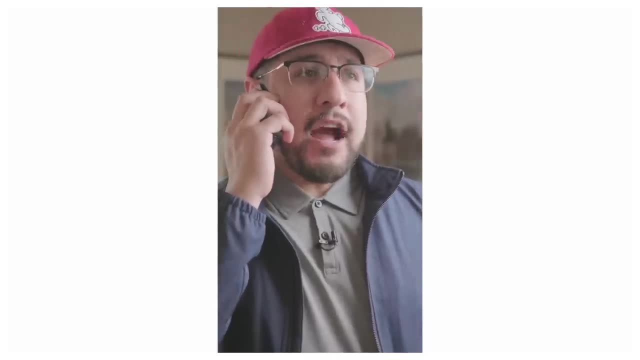 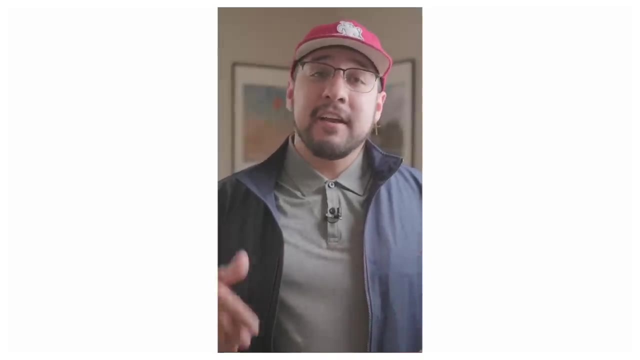 I can't put my photo side-by-side with this guy, Because you got me side-by-side with Larry the frickin' Lop. Listen, it shouldn't matter your body type, your height. What should matter is you having amazing, fantastic, well-built clothing that makes you feel like a stunner every time. 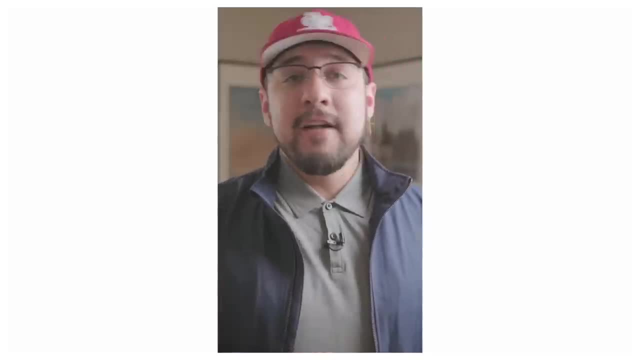 you step out And Cuts clothing not only makes a fantastic treat for yourself, but it also makes an amazing gift for your body. So if you're a Cuts fan, I would love to hear from you. And if you're a significant other? So if you're shopping for a guy, gal, non-binary pal, make sure to use promo. 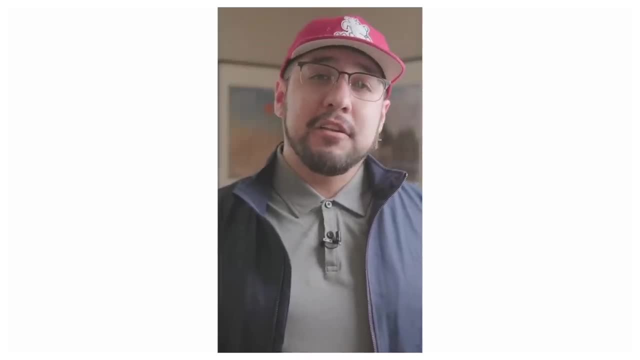 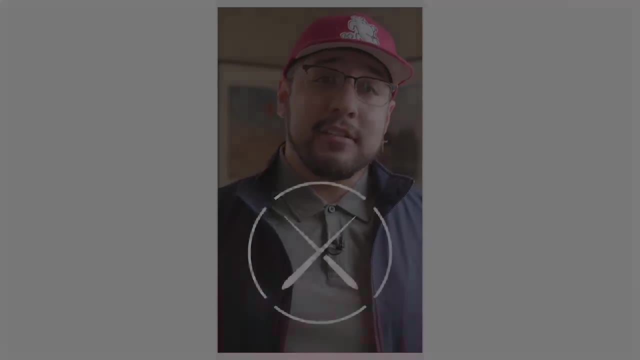 code DROSAFOTO to get 15% off your next Cuts clothing purchase. Listen, amazing, fantastic, well-built clothing that makes you look great should be for everybody, And it is. with Cuts clothing, I keep thinking: am I going to sell this, Am I going to keep it? And every time I